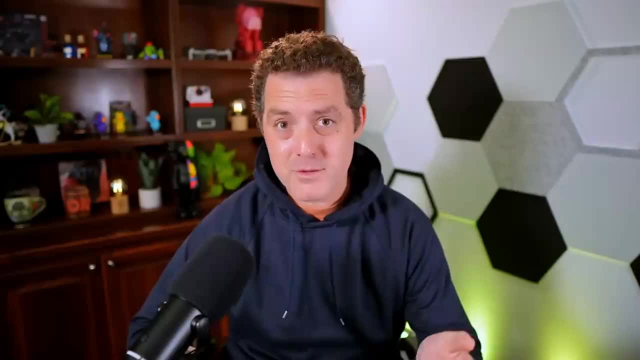 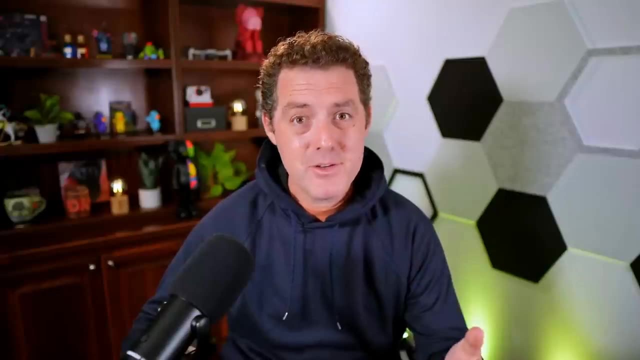 the setup couldn't be easier and they support a bunch of models with an increasing list, and you can bring any models that you want Plus. soon you'll be able to fine-tune your own models with this and you could use tools with this like Langchain and Hugging Agents. So I'm going. 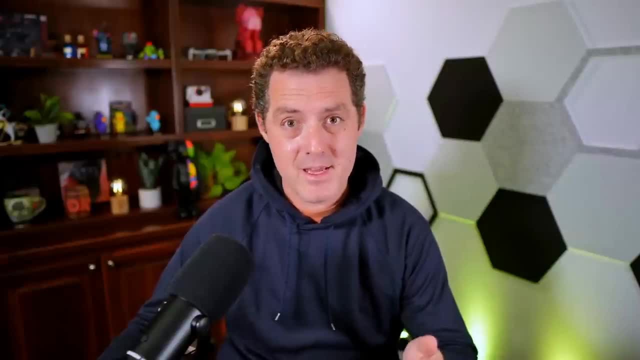 to show you how to install it. I'm going to show you how to get it set up and how to use it. Let's go. This is the OpenLLM repository page. I'm going to drop a link in the description below. 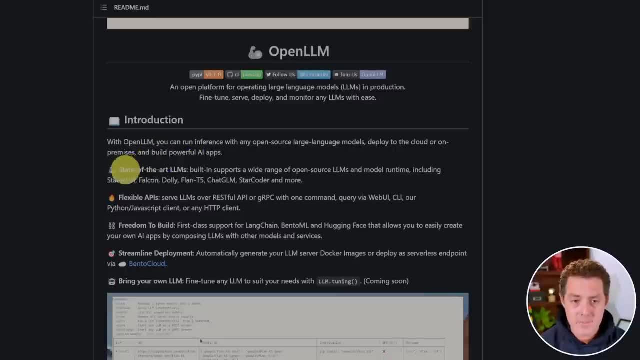 It is well documented already. Here are a few things they talk about State-of-the-art LLMs. they already support out-of-the-box StableLM, Falcon, DALL-E, Flan, ChatGLM, StarCoder and more. They also have super easy-to-use APIs that you can test using an interface. 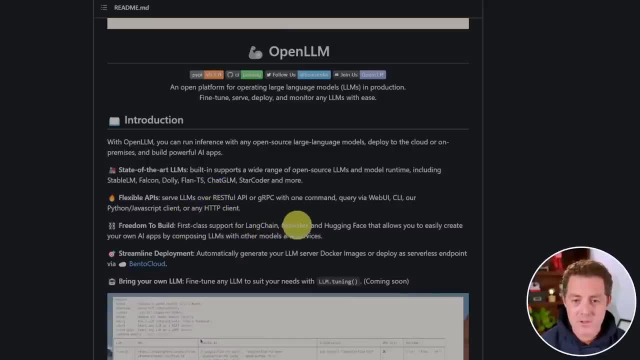 They also have first-class support for Langchain Bento LM Hugging Face, which you can use Hugging Agents and you could put together multiple different LLMs, which is nice. And here it says you can automatically generate your LLM server Docker images or deploy as a. 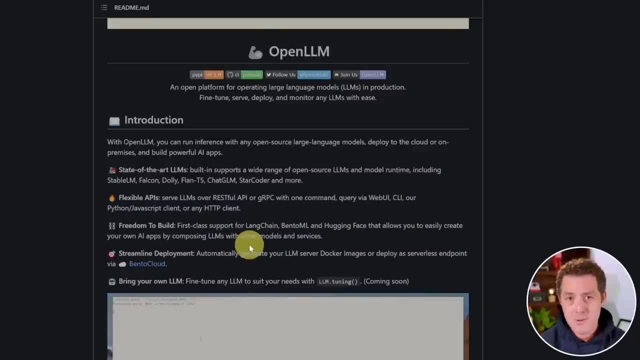 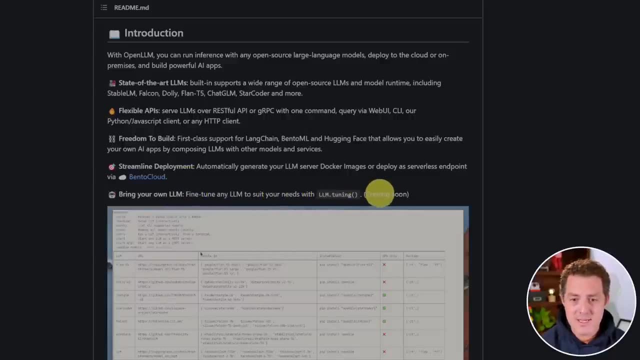 serverless endpoint via Bento Cloud, So super easy to go from local deployment to production ready And last, fine-tune any LLM to suit your needs. and that is a coming soon feature. First, let me show you how to get it installed. It's really only one command, but we're going to be using 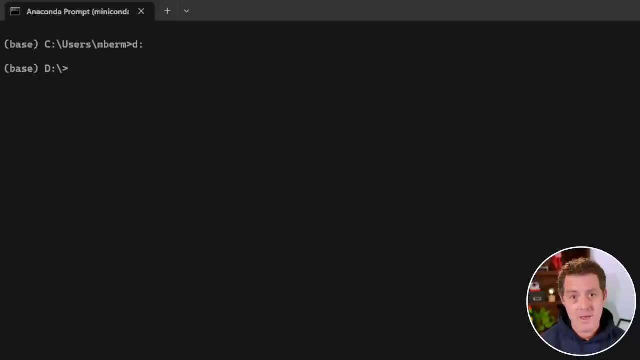 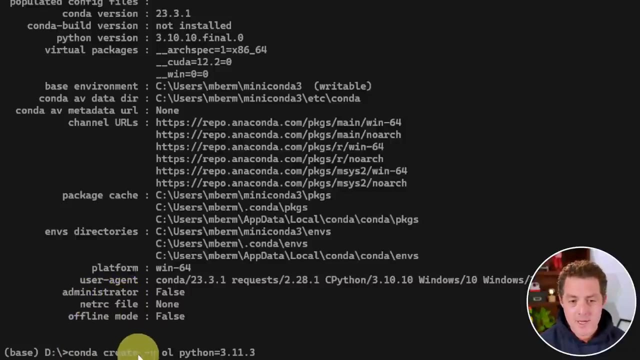 Conda, like we usually do, to avoid any Python and module mismatch issues, And the first thing we're going to do is create our new Conda environment. To do that, we're going to type conda: create dash n for name OL, which is open LLM, but you can name it anything you want. 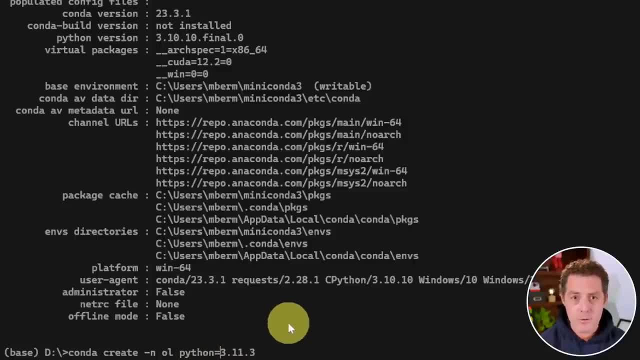 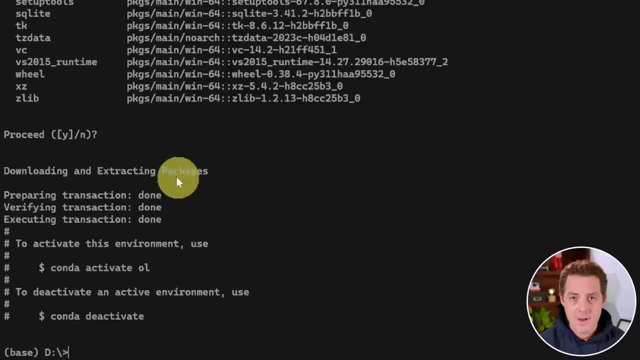 Python equals and we're going to be using Python version 3.1.1.3,, which is a very recent version. Then we hit enter. And here we hit enter again to say we do want new packages installed. All right, that's done. Now we activate the environment. We can just highlight this code: 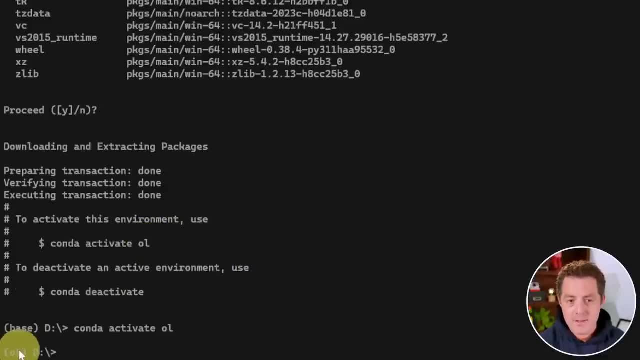 right here, copy paste it, and now we're activated. And we can tell that this environment is activated because it says OL right there. And now watch how easy this is: Pip install, open LLM. That's all you have to type. Enter. It installs everything we need. All right, it's done. 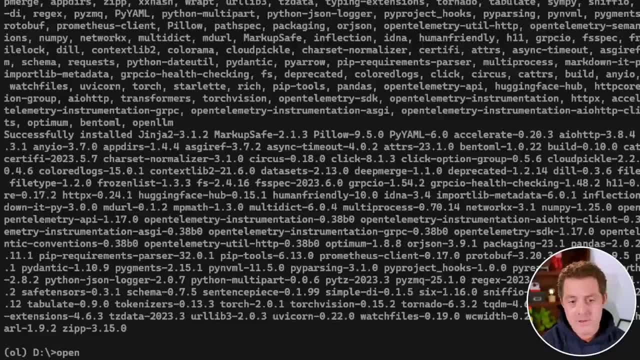 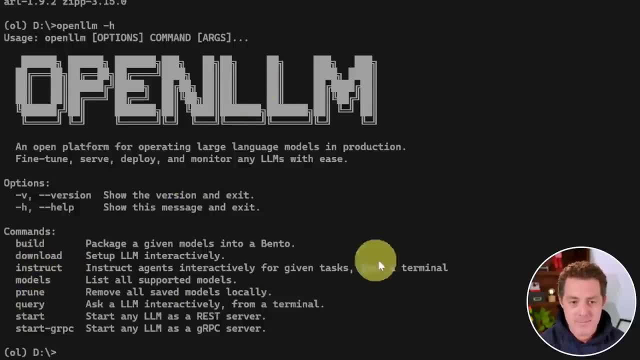 Now, to verify that we installed everything properly, all we have to do is type open LLM, dash h, And there we see that we have it available, and it tells us everything we need to know about the commands. Now, right here, it says start, and that allows us to start any LLM. 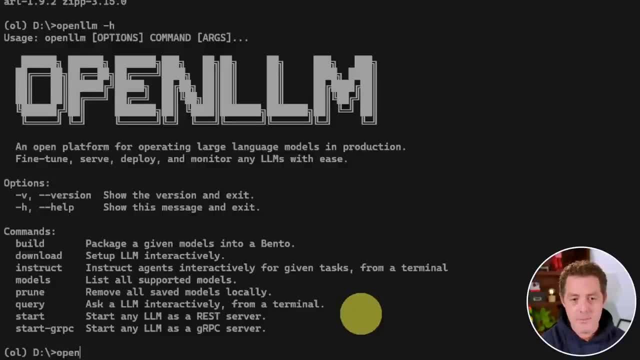 as a rest server. So to do that, we type open LLM- start, and then we're going to be using OPT, which is the one that comes out of the box with open LLM, But I'll show you how to install other. 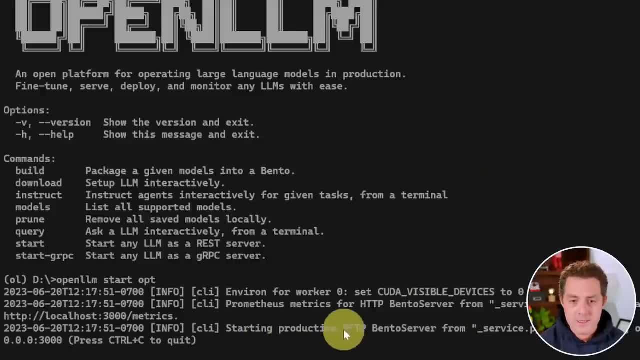 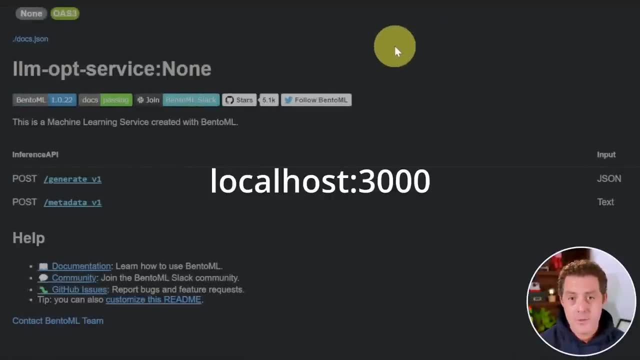 models as well. We hit enter and it's done, And we can see that the server is up and running And the only thing we have to do now is go to the interface, which is localhost, colon 3000.. And this is what it looks like. It's. 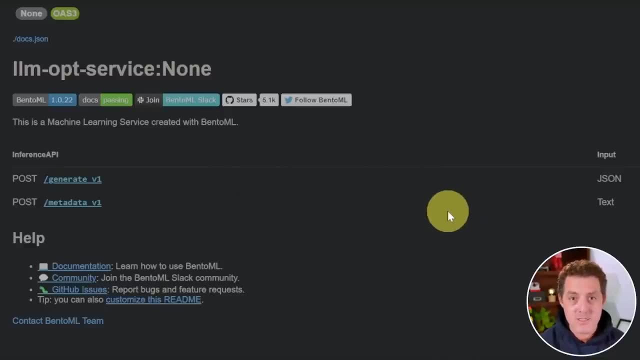 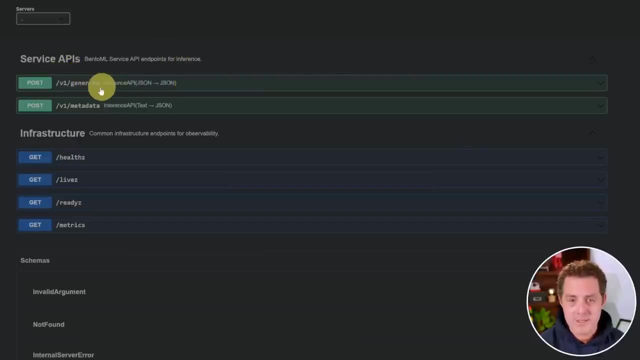 basically an API documentation page, But it also allows us to test the endpoint, which I'll show you right now. So if we scroll down a little bit under the service APIs, there's only two API endpoints that we really need to worry about right now. One is the generate. 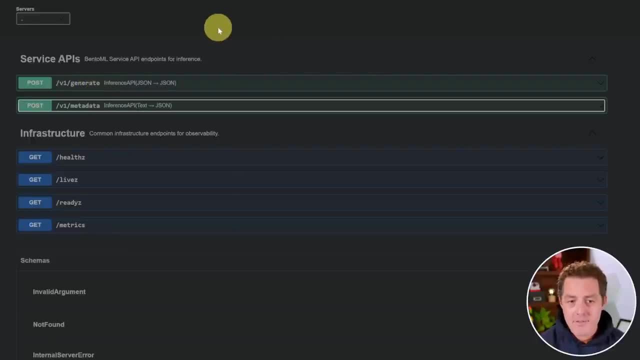 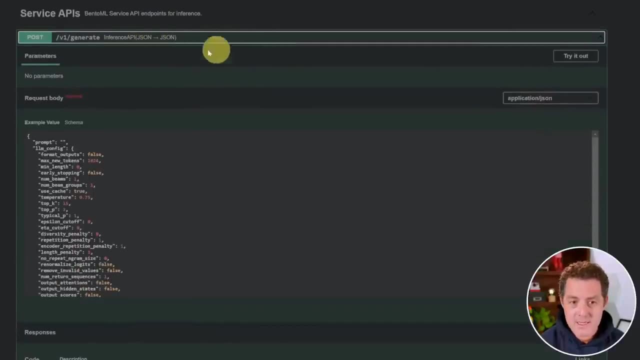 endpoint, which is going to be obviously the most frequently used, And then we have the metadata endpoint, which gives us additional information about the models and the server. So let's try the generate endpoint. So we just click that it opens up. we click, try it out And then right here. 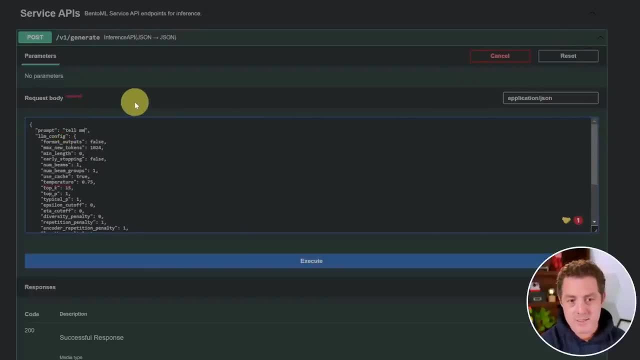 in the JSON. we're going to enter a prompt, So we're going to say: tell me a joke. then we hit execute And if you can just imagine this as an API endpoint, that's all it is. So we just pinged an API with this payload And we're waiting for the response. 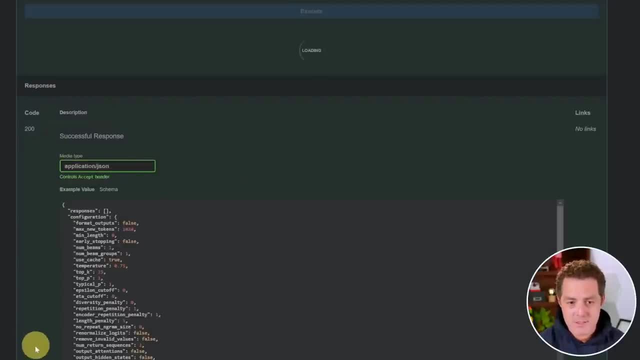 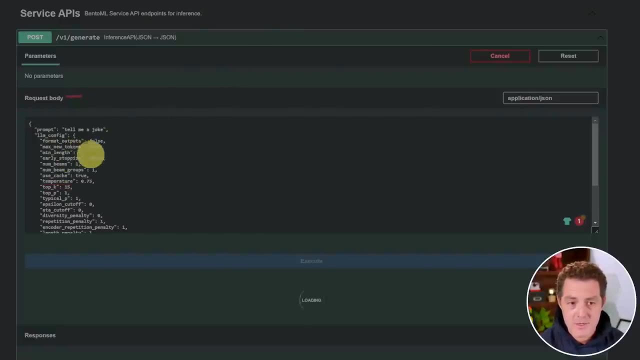 now And if we scroll down a little bit it tells us all the types of responses and the response codes that we can expect And keep in mind. as this is running, you can change all of these settings in here. So max, new tokens, min length, early stopping- it has a bunch of very common 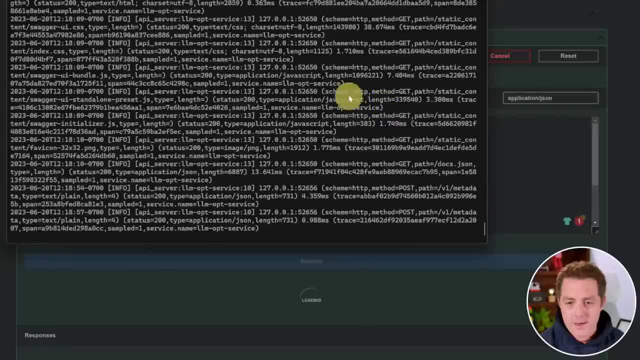 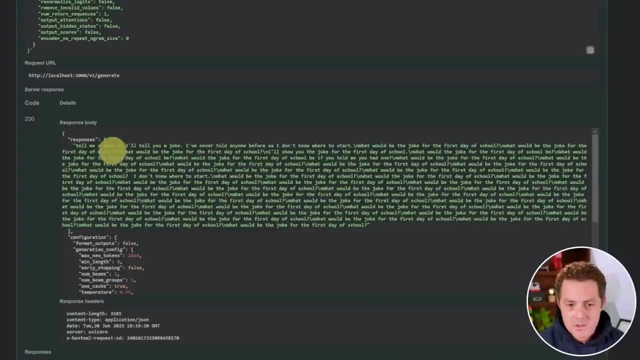 settings that you would expect with these large language models. And if we go back and look at our server, we can actually see that it is pinging the endpoints that we expect. All right, it's done, So we can scroll down. we can see the response here, Obviously, 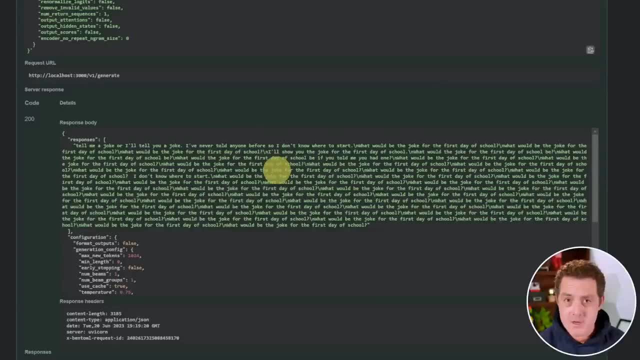 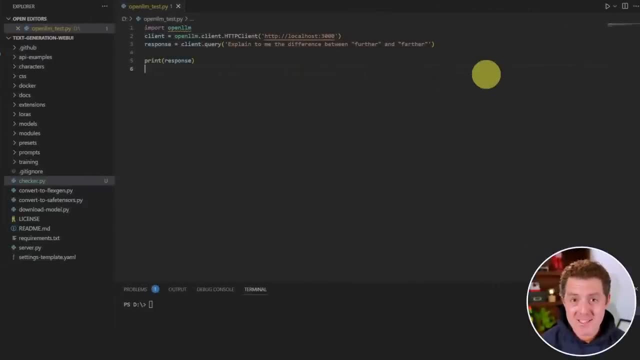 this response doesn't make a lot of sense, But that's only a reflection of the model- And this is a very small model- that we're using. Next, let me show you actually loading this into a Python application and how easy it is. So we still have that server up and running. And now what I did is: 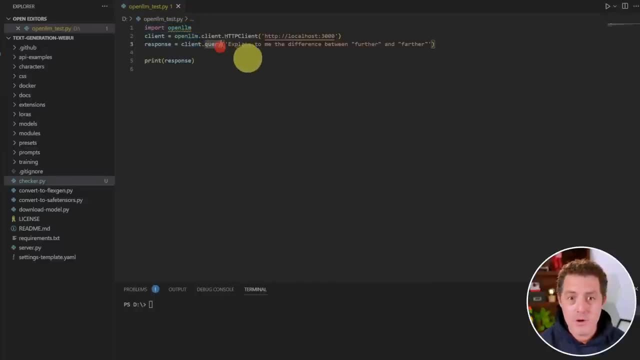 created this short Python script. So all we do is import open LLM. then we have the open LLM client pinging our local server And then here's our query. So I assign the response to this variable response And then I'm going to print it out. Now, let's run it top right. I'm going to hit play Now. 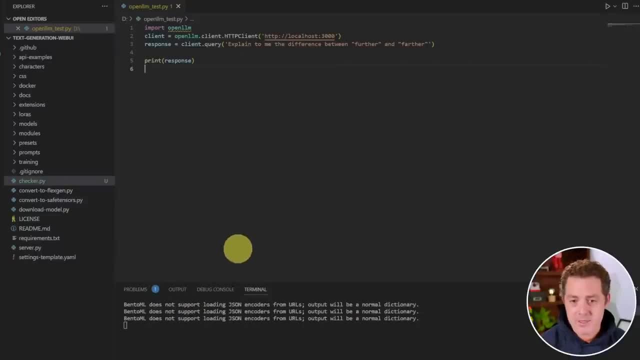 I get these warnings. bento LM does not support loading JSON encoders from URLs. output will be normal dictionary. I don't actually know what that means, But it doesn't seem to be causing any problems. And here we go. Explain to me the difference between further and farther, I think. 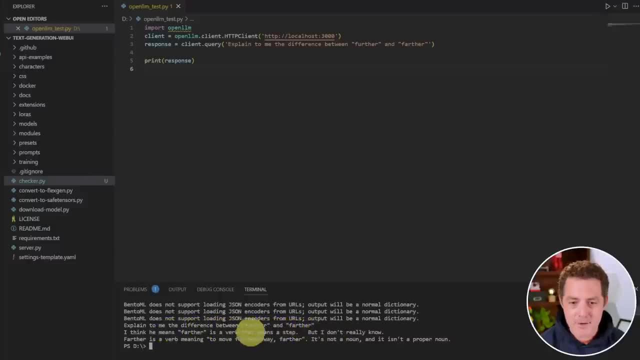 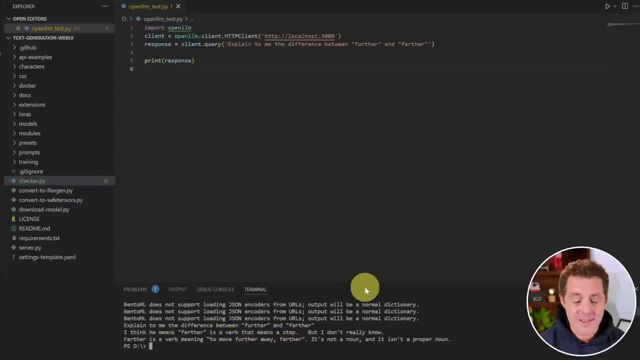 to print this out, And then I'm going to print this out, And then I'm going to print this out. Farther is a verb meaning to move further away, farther. Yeah, so the response doesn't make sense, But the API is working perfectly, And so just imagine you can put this simple code into any Python. 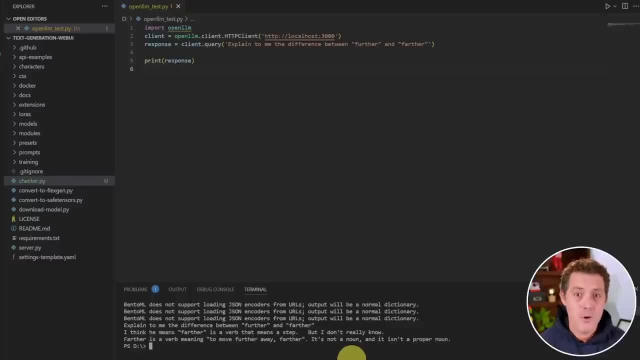 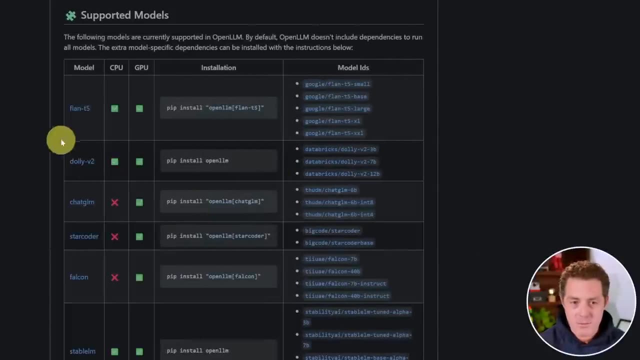 application that you want And you're going to have access to, building on top of an open source model that easily, And you can deploy the whole model really easily as well. So out of the box open LLM supports these models: flan, Dolly, chat, GLM, star, coder, Falcon, stable LM. 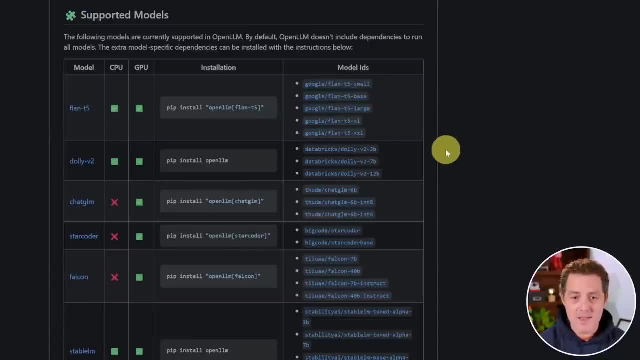 and multiple different versions of each of them as well. They could not be more easy to install. you just do pip, install open LLM brackets and then the model name. So let's try that out. Now I'm going to show you how to do that, So let's grab the. 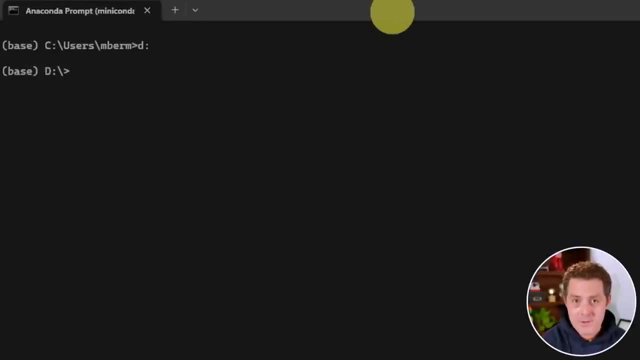 Falcon model. I'm going to copy that. I've opened up a new terminal while I still have that server running And of course I'm going to enable that conda environment. And now we have that same conda environment ready to go. So now we just do pip, install, open LLM Falcon and I'm going to hit. 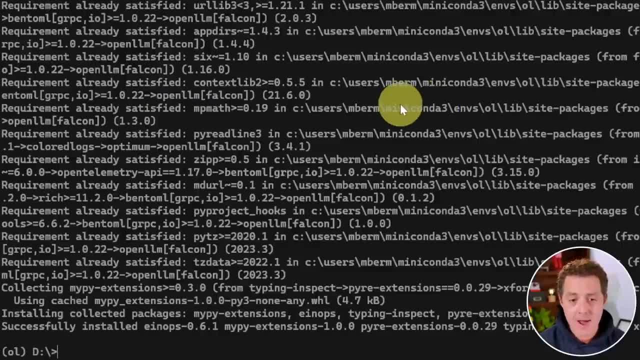 enter. Okay, so that worked. Now, one thing to note is I've gone through this installation before and the first time I did it it gave me some warnings. at the top It said: please make sure you have installed, and it gave me three or four different modules that I needed to have installed and it 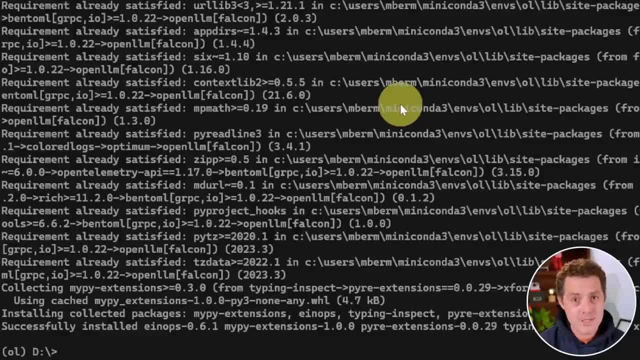 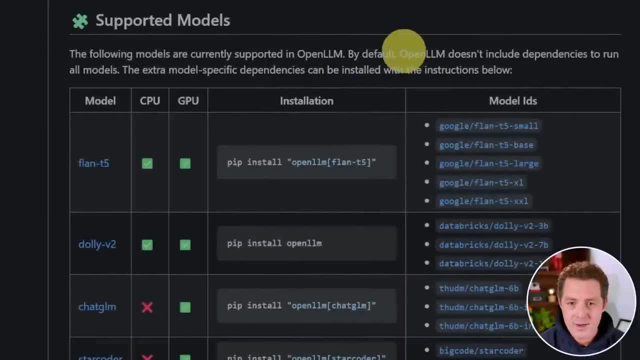 failed the first time, then I simply did pip install for each of those modules And then it worked And it tells you upfront what you need to install. So just keep that in mind, And it says it right here: Open LLM doesn't include dependencies to run all models, And so that's what you're going. 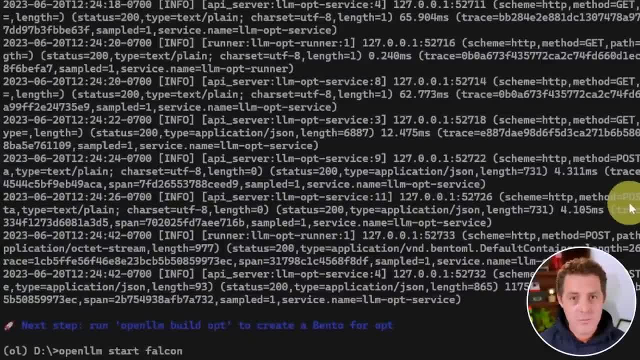 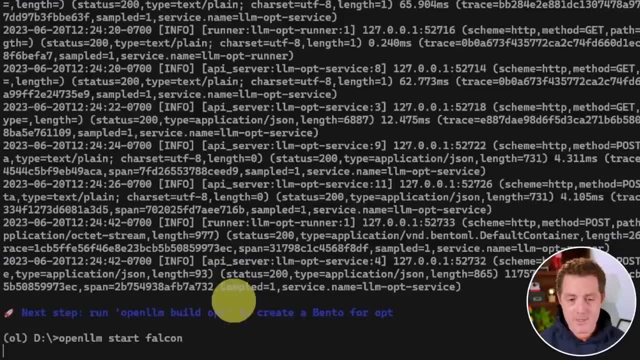 to need to install, But again it tells you. so now to run the model that we just installed, we've spin up a new server, open LLM, start and then Falcon instead of OPT. then we hit enter, Okay. so here's that warning I was talking about. make sure to have the following dependencies available: 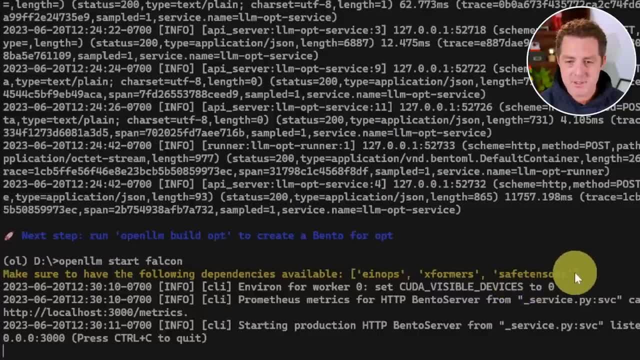 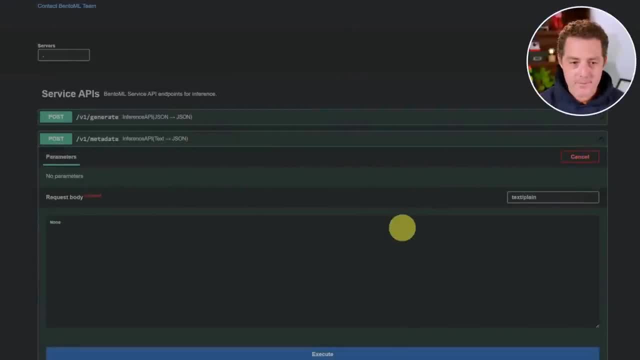 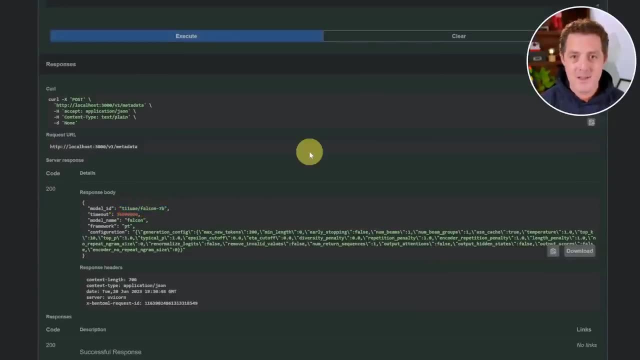 EIN ops X formers and safe tensors. Now, I already have those installed, but you might have to do that. And now, if we go down to the metadata endpoint, let's try it out: Execute, And here we go. We're using Falcon 7b. Now how awesome is that. So this is so easy to. 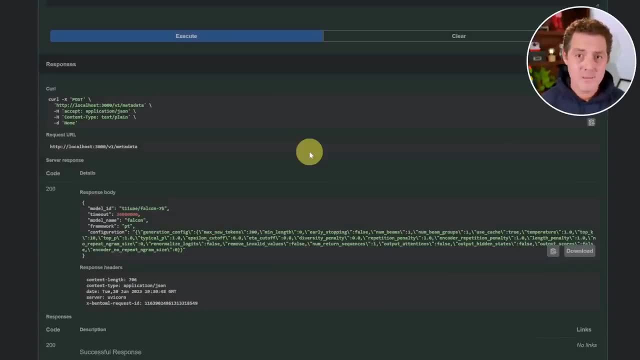 do. I'm so excited for this project because one of the biggest limiting factors of using open source models as an engineer was how difficult it was to build on top of them. But now this is a dead simple interface for building on top of these open source models. Okay, so now let's say I test. 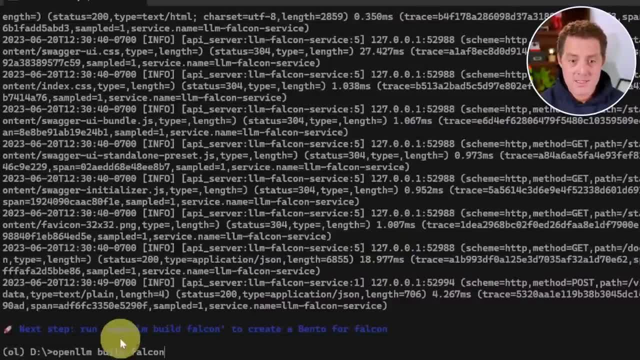 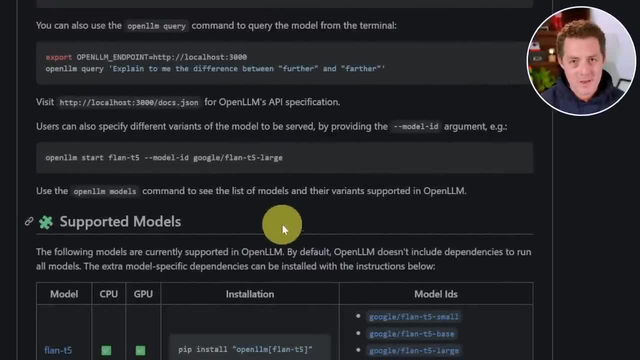 it out, all my code and I'm ready to deploy. all I would need to type is: open LLM, build Falcon, and then I just hit enter And that's going to create a bento. Okay, a couple last minor things. One: 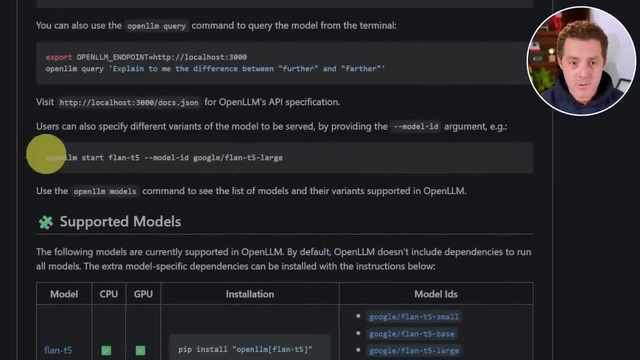 you can specify different versions of open LLM build Falcon. and you can specify different versions of open LLM build Falcon. and you can specify different versions of open LLM build Falcon. and you can specify different versions of models with this simple command: open LLM- start, and then you 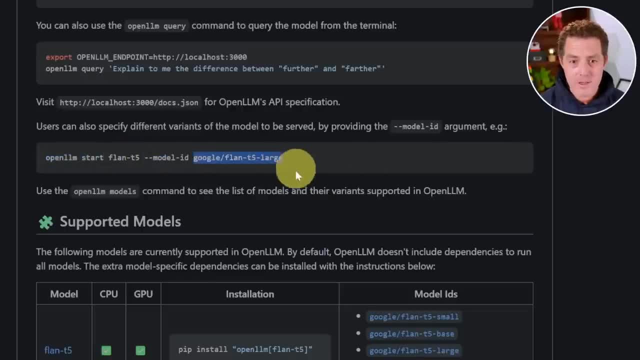 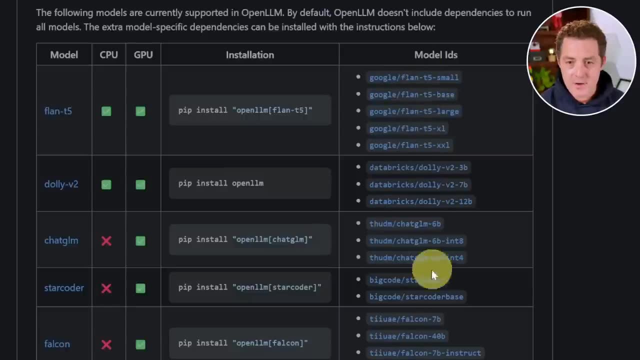 list the model and then you say model ID and then you put the model ID at the end, And that will make it so that you're actually starting the server with a specific variant of a model. And here you can see all the different variants of the model. And, as I mentioned at the beginning, 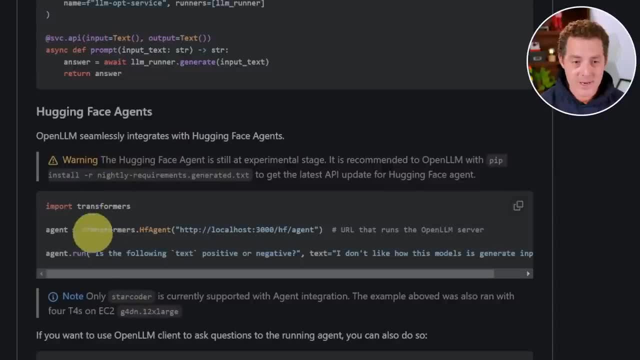 they also have a Hugging Face agents integration already, So you can use Hugging Face agents with any of these local models. So you're really talking about extremely powerful tools now being available completely open source. So you're really talking about extremely powerful tools now. 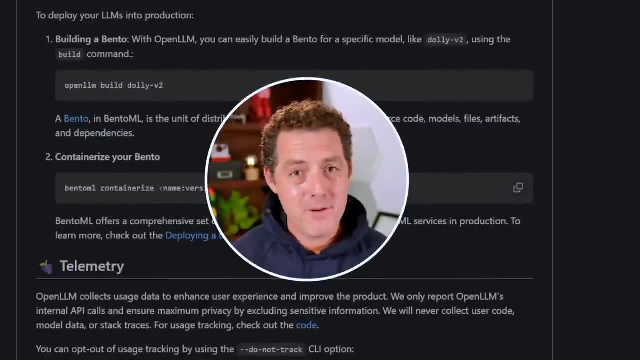 being available completely open source. So you're really talking about extremely powerful tools now being available completely open source. So you'll see that this is going to be simply a question of how it does and how it's using my properties. that will be protected by those miracles of useful things And if you're free to do that, that's nice, Right. I'm not giving instructions on some of the other things today which are probably going to be about. 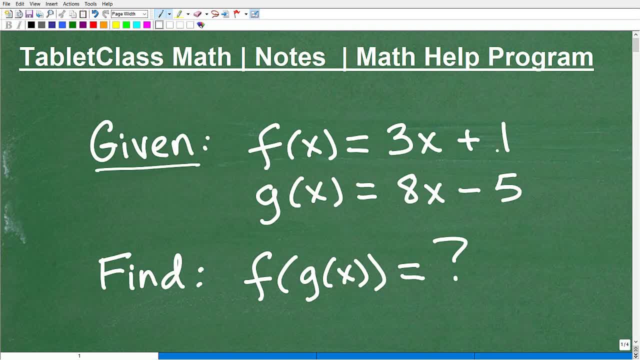 Okay. so given f of x is equal to 3x plus 1 and g of x is equal to 8x minus 5, I'd like you to find f of g of x Okay, and hopefully most of you out there recognize that the topic of this video is composite functions.